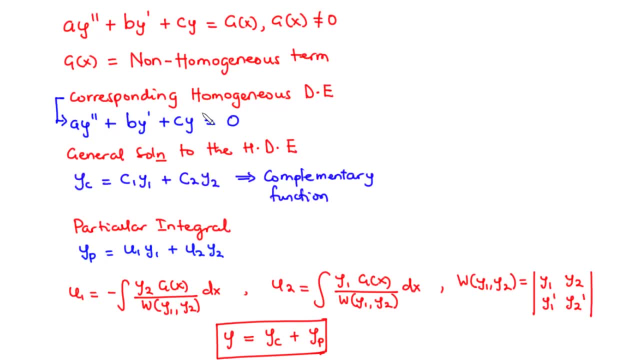 thing is to find the general solution of the corresponding homogeneous differential equation, and that is given by: yc equals c1 times y1 plus c2 times y2.. Now this function is what we call the complementary function. So this is the general solution with respect to the corresponding 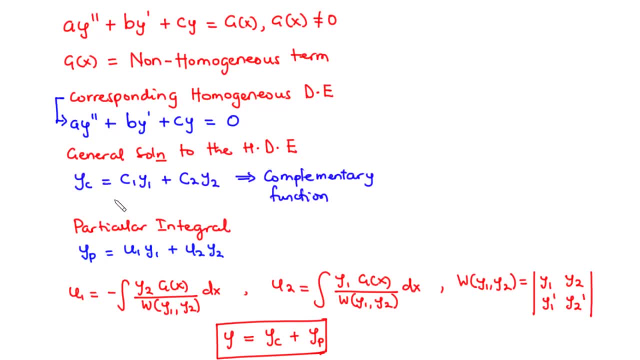 homogeneous differential equation. Now to find the particular integral or, better still, the particular solution. what we are going to do is to vary the parameters, that is, by replacing the constants c1 and c2 in the complementary function and then replacing them by u1 and u2 respectively. Now notice that u1 and u2. 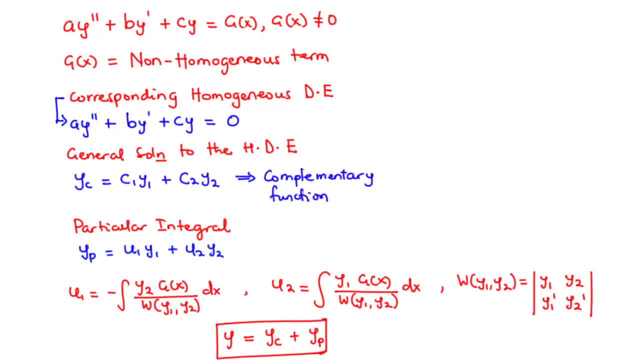 are functions of x, They are, better still, unknown functions of x, and we seek to find the functions u1 and u2.. Now, u1 is giving us the negative integral of y2 times g of x, divided by the wrong scan of y1, and 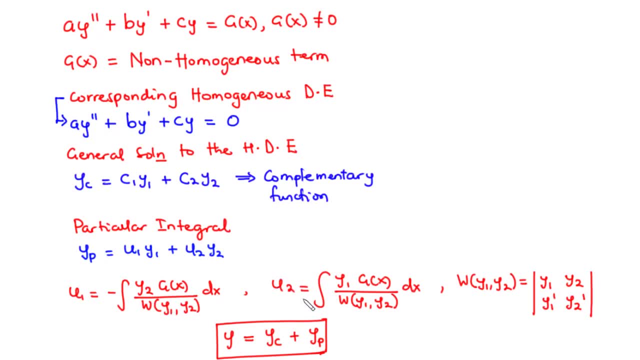 y2, the x, and then we have u2, also giving us the positive integral of y1 times g of x, divided by the wrong scan of y1 and y2, the x, and the wrong scan of y1 and y2, because we are talking about two. 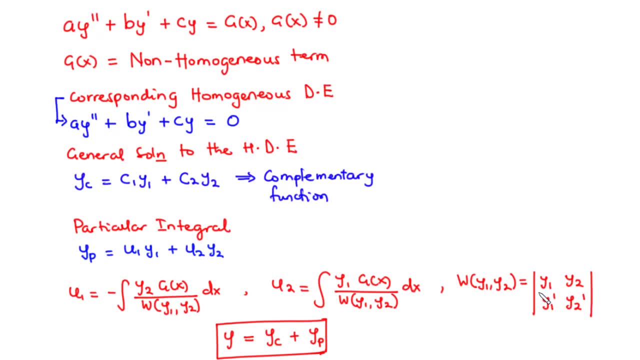 functions here. So in the first row we have it occupied by the functions themselves, so y1 and then y2, and the second row is occupied by the first derivatives of y1 and then y2.. Now at the end you have the particular solution or the particular integral to be. 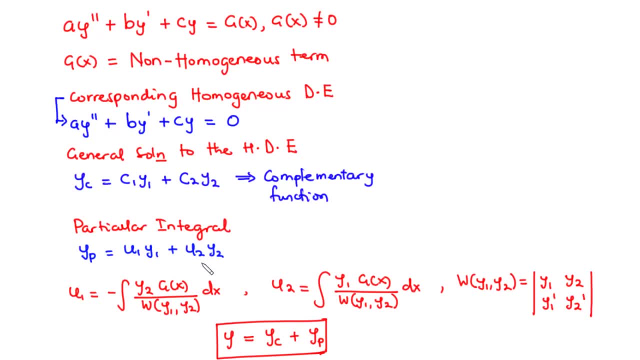 yp equals u1 times y1 plus u2 times y2, and thus to find the general solution to the given differential equation, you basically add the two solutions, yc and then yp, to get the general solution to the non-homogeneous differential equation. so in this lesson we are going to solve three examples. let's 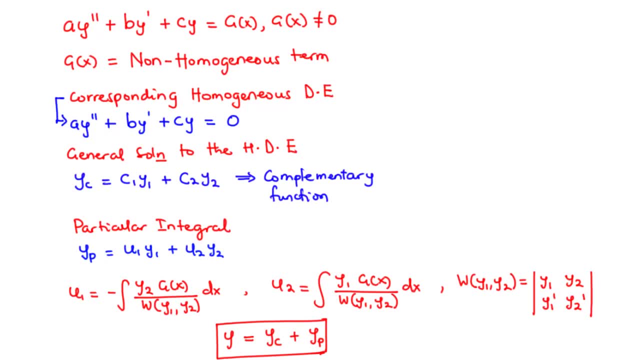 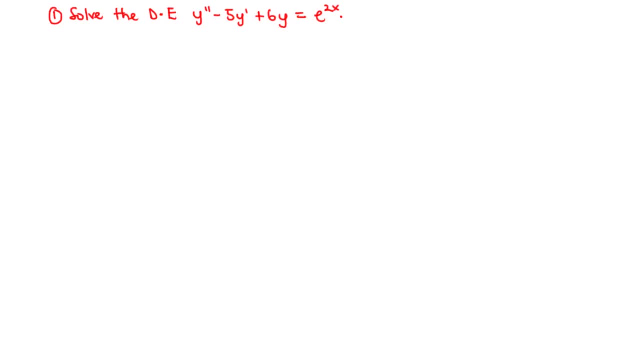 start off with the simplest of examples. so, for example one, we are going to solve the differential equation y prime prime minus five, y prime plus six. y equals e to the power two x. now this is a familiar differential equation. so let's try to solve this differential equation together and 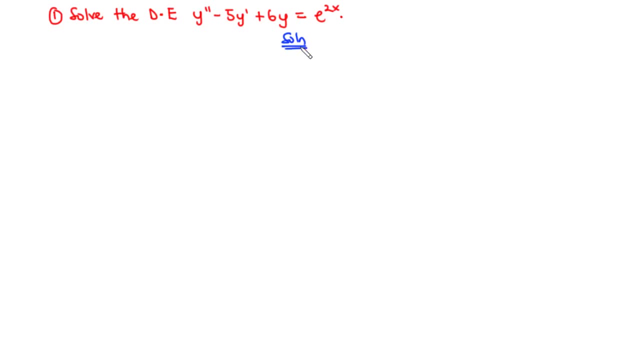 notice that we are going to use the method of variation of parameters. so we have the differential equation: y prime prime minus five, y prime plus six, y equals e to the power two x. so first of all we are going to generate the corresponding homogeneous differential equation from this, so that is given by y prime prime minus five, y prime plus six, y equals zero. 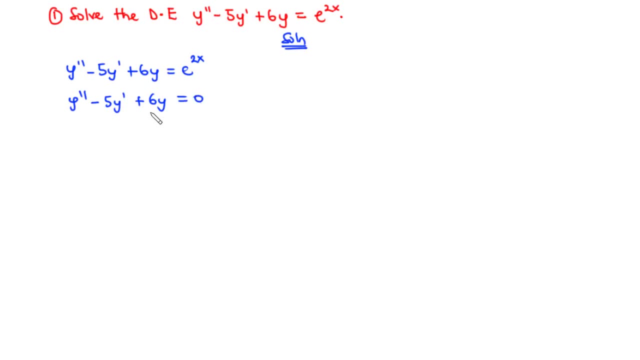 and then we are going to derive the auxiliary equation from this. so we have m square minus five. m plus six equals zero. so let's try to find the factors. so we multiply the coefficient of m square, which is one times coefficient of constant, which is six. so one times six is six. we need to generate two numbers that when you multiply you have six. 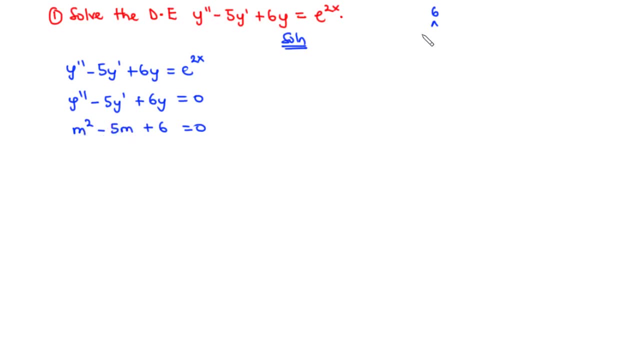 when you add, you have negative five. so we can talk of negative one, negative six and then negative two, negative three. so we are going to select these two values now. negative two times negative three is six. negative two plus negative three is negative five. so we have m minus two, and then m minus three equals zero. 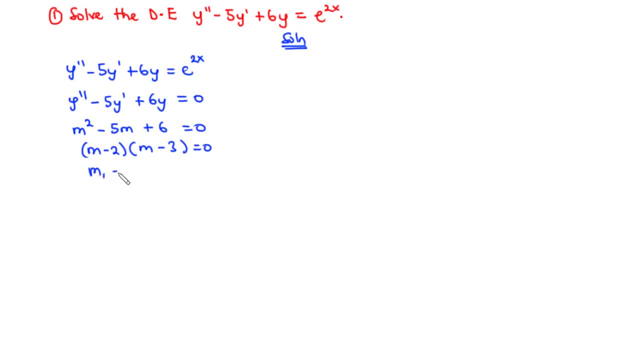 so we have m 1 to be equal to two and then m 2 equals 3. therefore, the general solution to the corresponding homogeneous differential equation or the complementary function is given by c, 1 plus n, 3 plus 3. eternal error. but if we wanna talk about n1 and then n2, can we just be using both of these. we need to have n1 and then n3 equals n3 equal to. 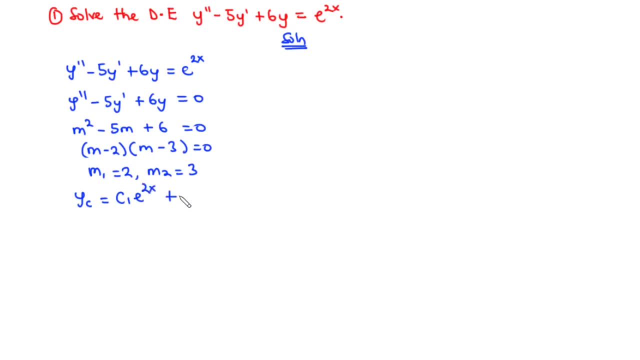 1. equivalently, now and for theил term, we are using four, two, then two of these, so we have n, one plus negative three equals zero. soê 1: e to the power 2x plus c2 e to the power 3x. Now, at this point we have: 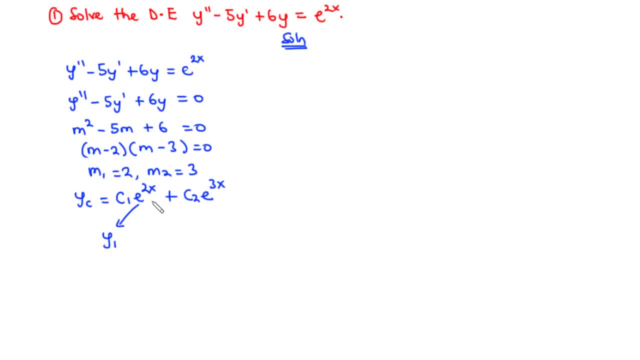 e to the power 2x to be y1, and then e to the power 3x to be y2.. So we have y1 to be equal to e to the power 2x, We have y2 equals e to the power 3x, and then we have g of x. 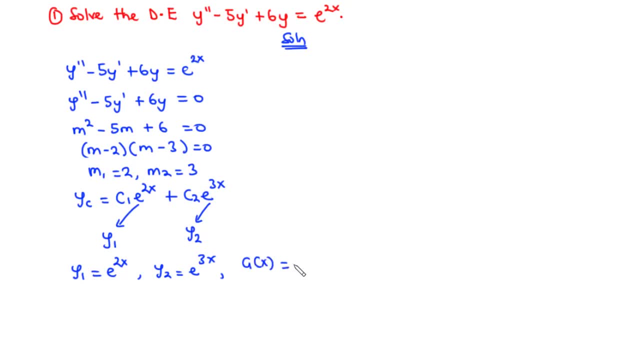 g of x to be equal to e to the power 2x. Now, since we've been able to find the complementary function, let's move on as we find the particular integral or betas to the particular solution. So we know that the particular solution is given by yp equals. 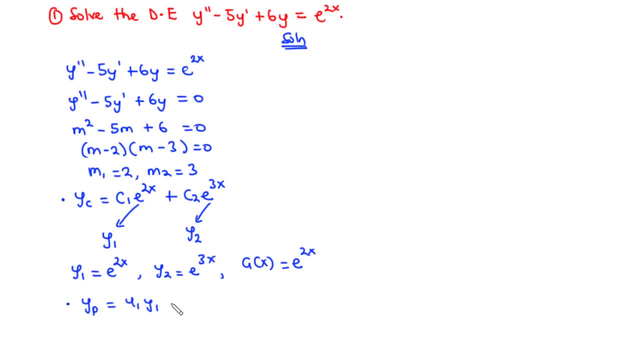 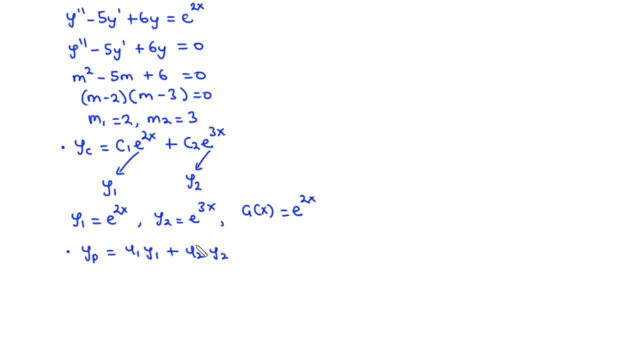 yp, u1, y1 plus u2- y2.. Now, before we can find u1 and then u2, we need to find the run scan of y1 and y2.. So we know that the run scan of y1- y2 is given by the determinant of. we have 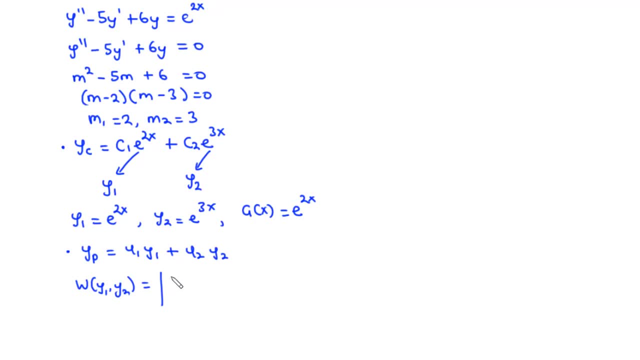 two functions, so the determinant of a two by two matrix. So thus we have y1, y2 and then y2.. y1 prime, y2 prime. So for y1, we have y1 to be e to the power, 2x, y2, e to the power. 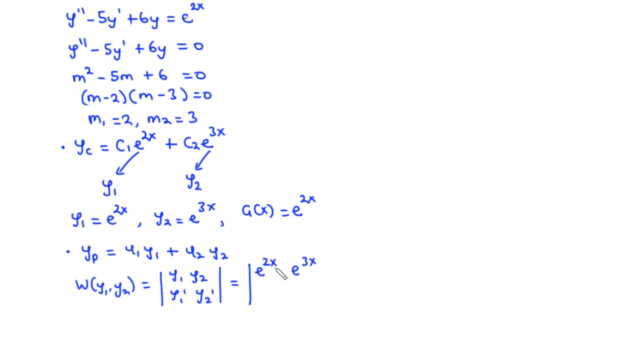 3x And then, if you want to differentiate this with respect to x, then you have 2 e to the power 2x And with this you have 3 e to the power 3x. Therefore, to find the, 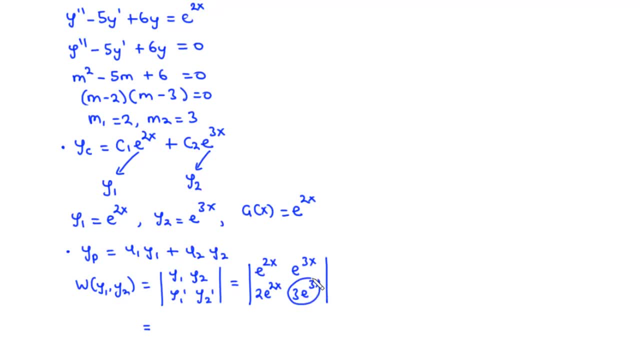 determinant. we multiply this value by that value, So we have 3 times 1,, that is 3, and then e to the power. here we have 2x, here we have 3x, So that's going to be 2x plus. 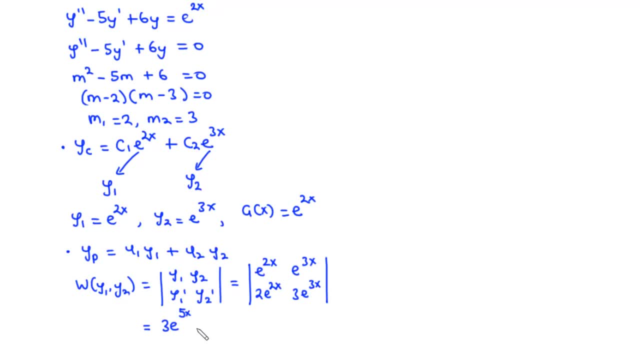 3x, that is 5x. So 5x and then minus. we multiply these two values. So 2 times 1 is 2, e to the power, 2x plus 3x, that also gives 5x. So basically we are going to have 3 e to the power, 5x minus. 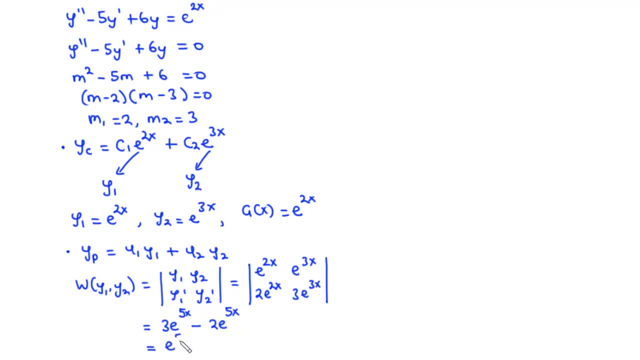 2. e to the power 5x. We are left with e to the power 5x. So this is the run scan of the two functions. So the next thing is to find u1 and u2.. So for u1, that is given by negative, the integral. 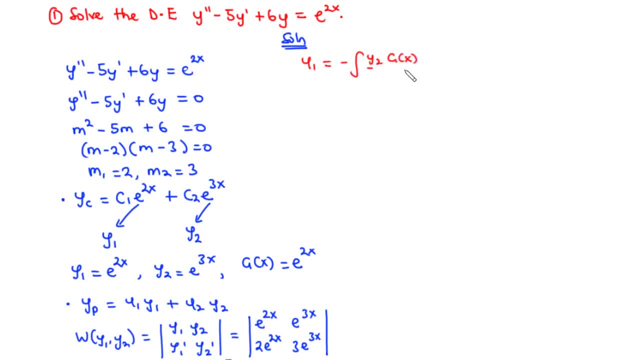 of y2 times g of x. So y2 is e to the power 3x divided by the run scan of the two functions. So we have negative the integral of. now y2 is e to the power 3x, So e to the power 3x times g of. 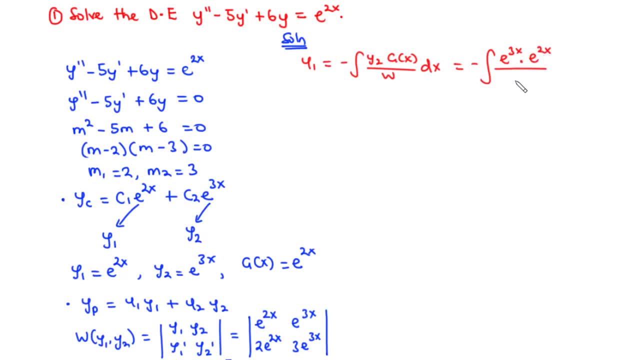 x, e to the power 2x divided by w, which is e to the power 5x. That is the run. scan the x. Now. e to the power 3x times e to the power 2x is equal to e to the power 5x. So 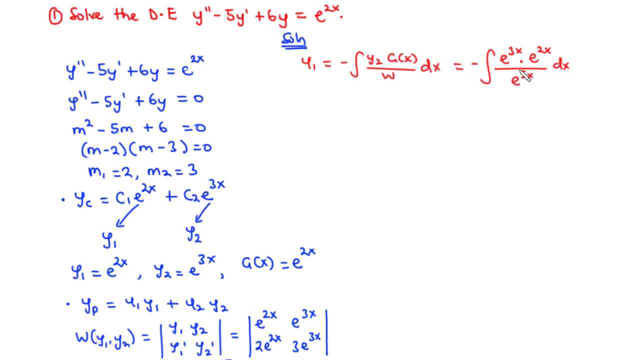 So e to the power 5x cancels out e to the power 5x, and then we are left with 1.. Therefore we have u1 equal to negative, the integral of 1, dx. Now if you should integrate 1 with respect to x, then that is equal to x. 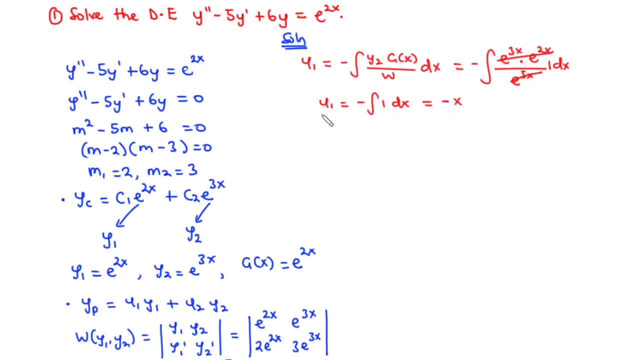 And then we have this negative attached to it. Now, because we are going to cater for the constant in the final solution, we are going to ignore the constant of integration. Therefore, we have the function u1 to be equal to negative x. 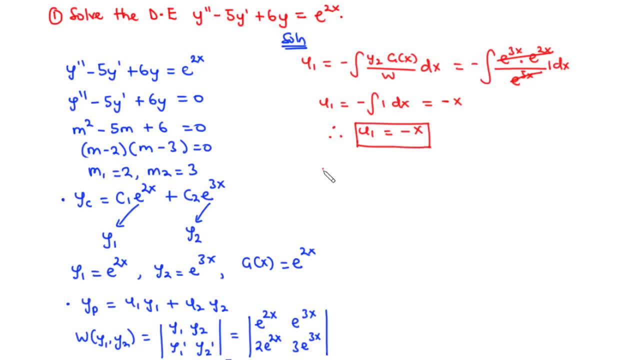 So that is u1.. Let's try to find u2.. So u2 is also given by the positive integral of y1 times g of x divided by the wrong skin, dx. So we have y1 to be e to the power 2x. 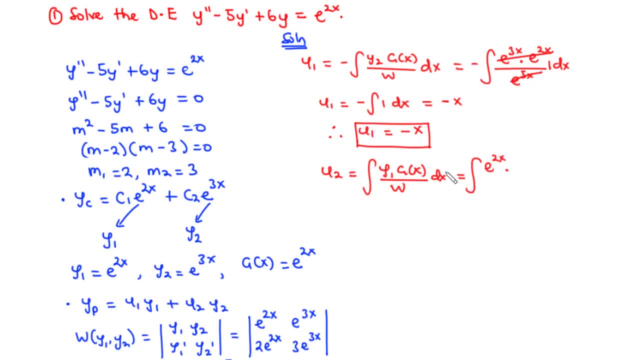 times g of x. also e to the power 2x divided by the wrong skin. e to the power 5x dx. So this becomes the integral of e to the power 4x divided by e to the power 5x dx. 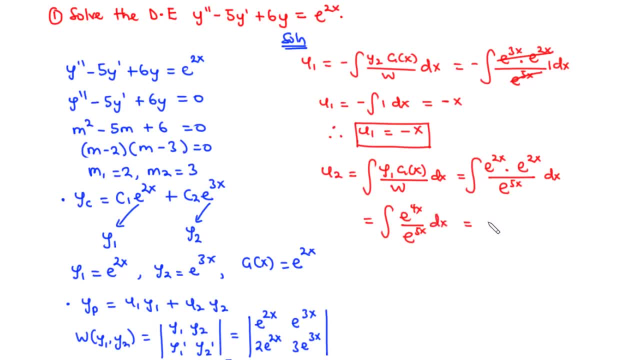 And that is equal to. We are going to have the integral of e to the power 4x minus 5x, And that is equal to e to the power negative x, dx. Now let's try to integrate this function. 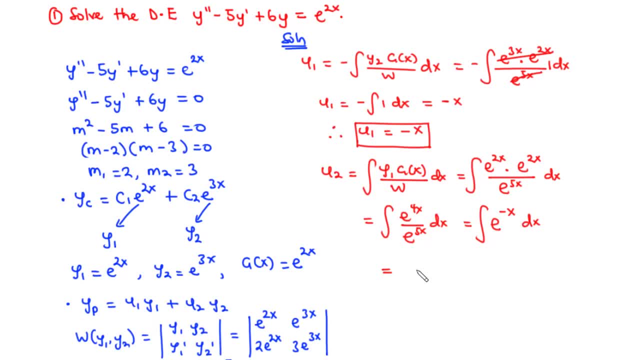 So when we integrate e to the power negative x, then we still have e to the power negative x, And then we differentiate negative x and that becomes negative 1. And that appears at the denominator. So naturally we are basically going to have: 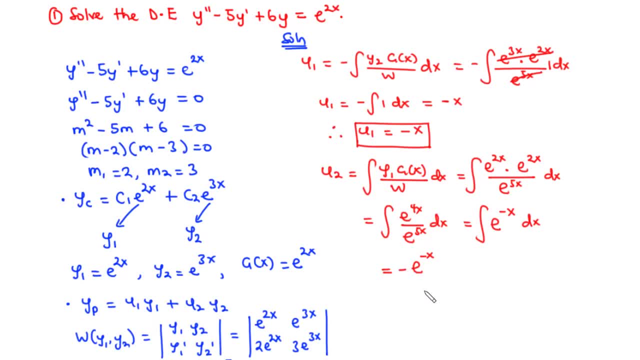 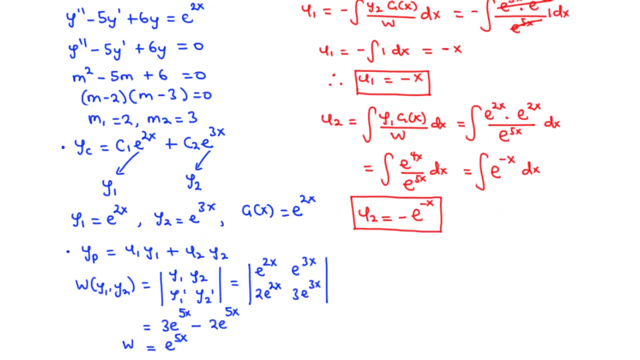 negative e to the power, negative x, So that is u2.. Now, from this, which is the particular integral, we have yp to be equal to u1.. So we have u1 to be negative x times y1, which is e to the power 2x. 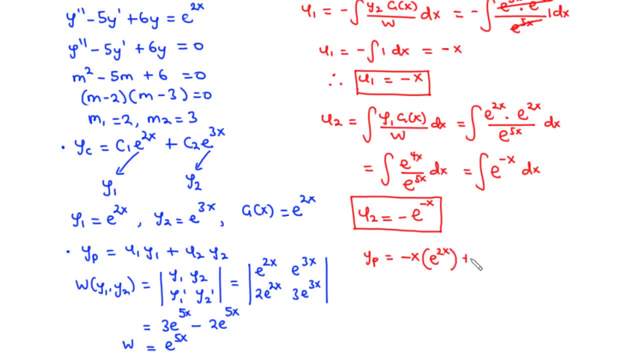 Plus u2, which is also negative e to the power, negative x times y2,, which is e to the power 3x. Now let's try to simplify this. So we are going to have negative e to the power 2x times x. 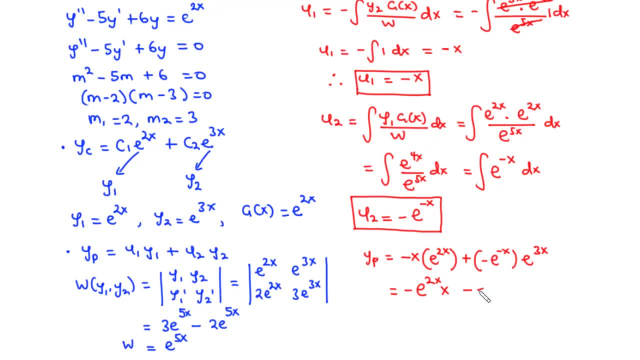 And then here we have minus e to the power, negative x And then plus 3x. So negative x plus 3x is 2x, So this is yp. Now let's try to combine the two solutions, which are yc and then yp. 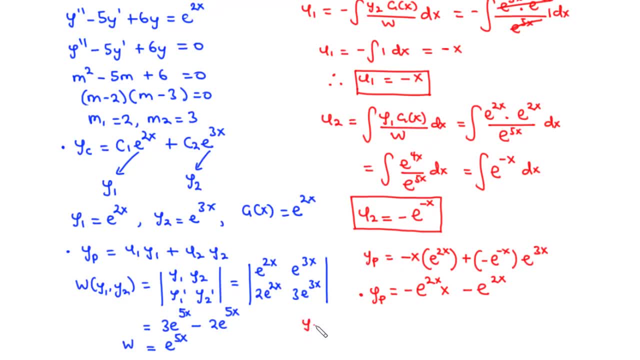 Therefore we have the general solution to the differential equation. y equals yc plus yp. So for yc we have c1 e to the power 2x plus c2 e, So we have c1 e to the power 3x plus yp. 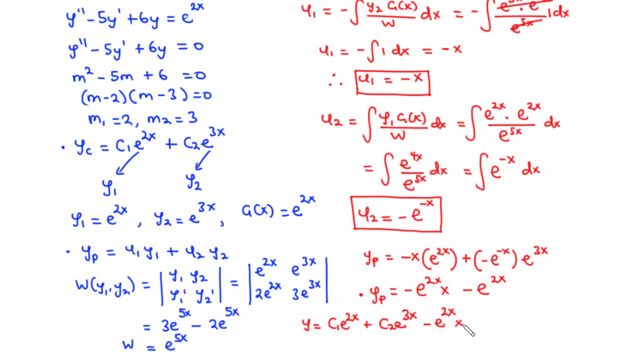 So negative e to the power 2x times x minus e to the power 2x. Now here we have e to the power 2x, e to the power 2x. The coefficient of e to the power 2x here is negative 1.. 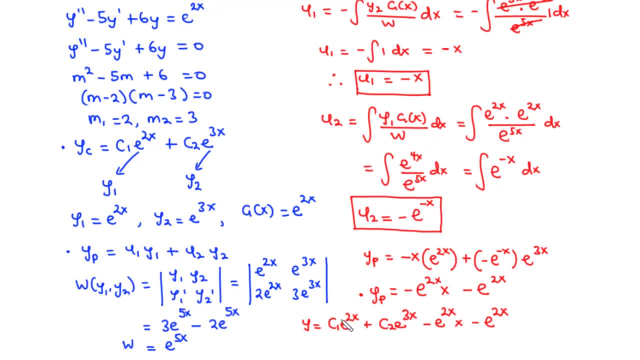 Coefficient of e to the power 2x. here is c1.. Now c1 and the negative 1 are all constants. So constants or a constant Minus a constant is still a constant. Therefore we can simplify this general solution so that we have y equals.